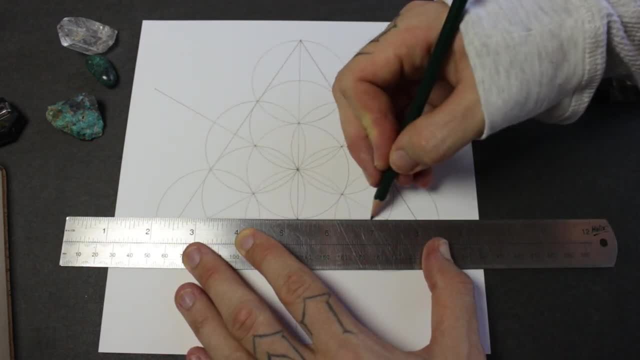 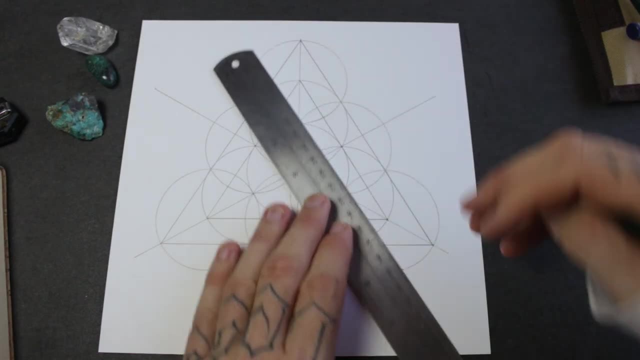 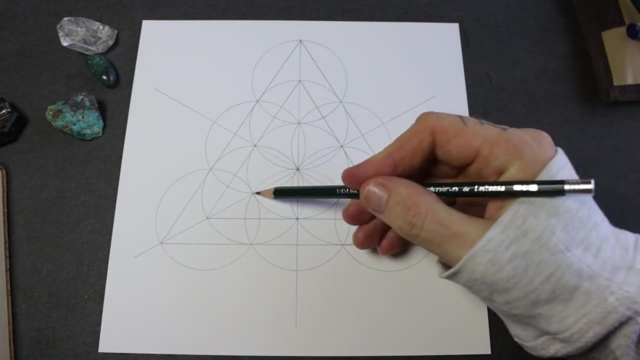 another triangle inside the triangle, So I'll do the same on these points as well. That one is cool because it's got the circle inside of it, which just looks pretty sick, And then now I'm going to use these points to draw another triangle. 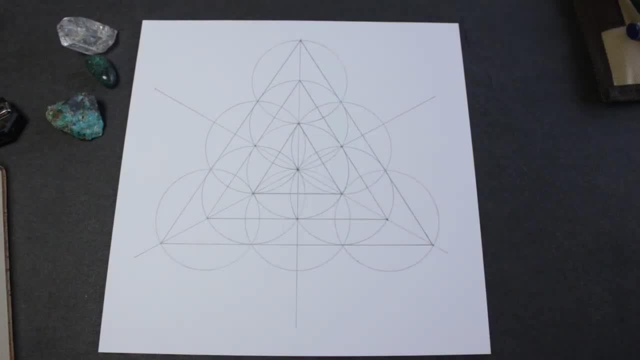 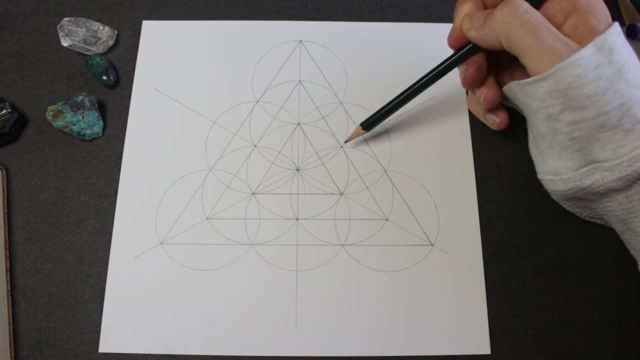 And now we've got three triangles inside the seed of life. And now what I want to do is I'm going to, I'm going to need, I'm going to need upside down triangles now because I want to make a hexagram in the center. 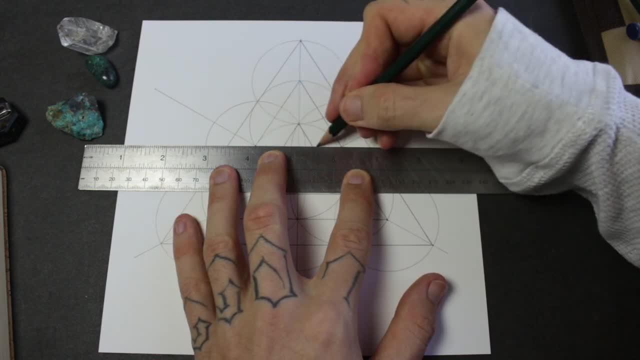 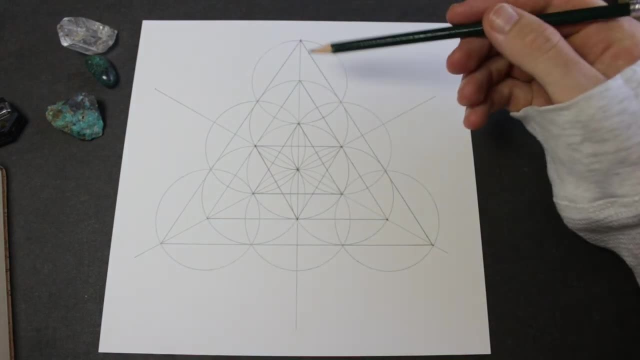 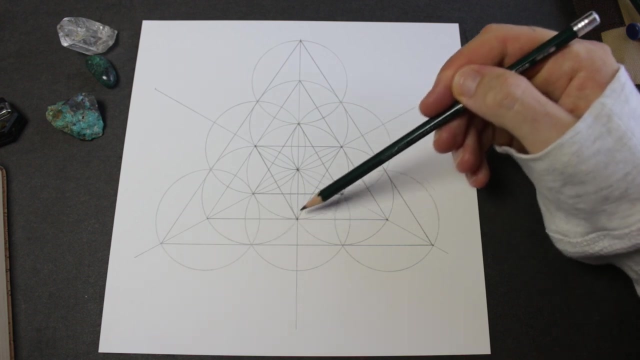 So I'll start off with the one in the middle: Hexagram in the middle. Okay, So if you look close, I got this circle is within the triangles, This circle is within the triangles, This circle is inside And this one is inside. 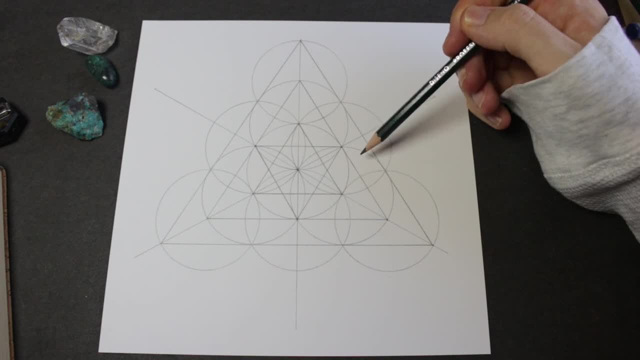 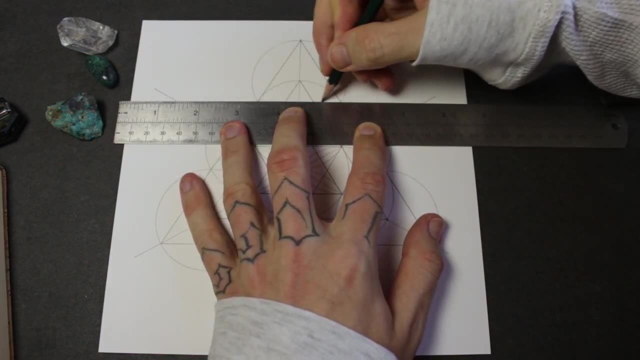 And those are the circles that I want to put hexagrams inside of. All of the rest, just forget about them, I don't even care. So that's. what I'm going to do is just put hexagrams inside of that The circle, inside the triangle. 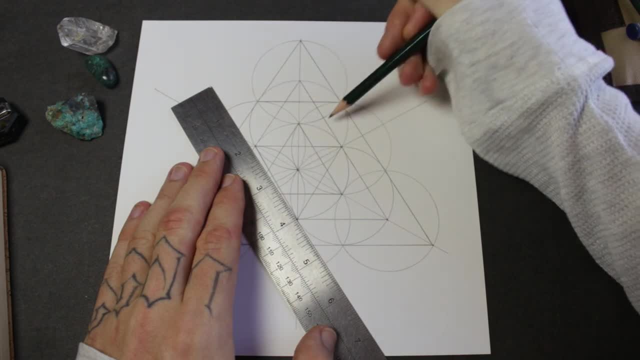 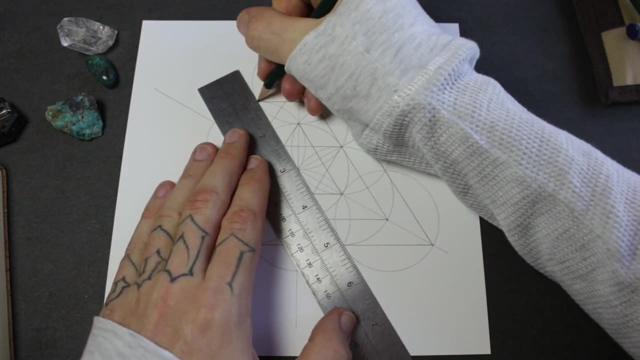 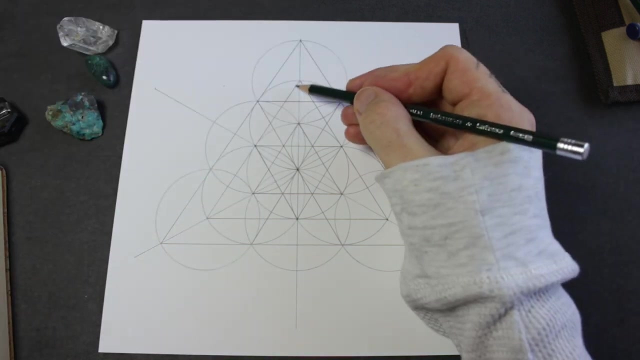 So this one would be: go down to here to make the upside down triangle. but we can actually just cut all the way through and then start making the triangle in the other circle as well. Do the same on the other side, And then you see we got the hexagram inside that circle. 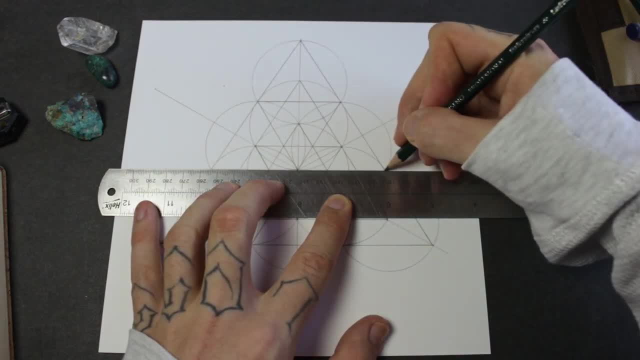 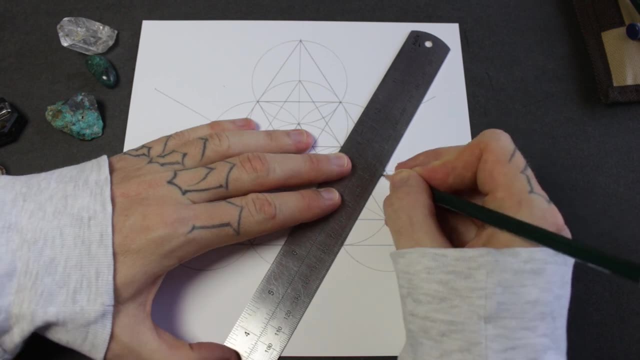 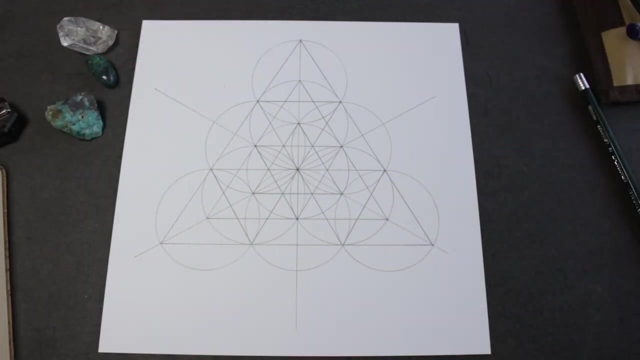 And then here. I can just go through there and then here, and then the last one will be here. There we go. We got four hexagrams inside of the big triangle and that's already looking pretty powerful in it. But to make it even more powerful, what we've got to do is around each one of those hexagrams. 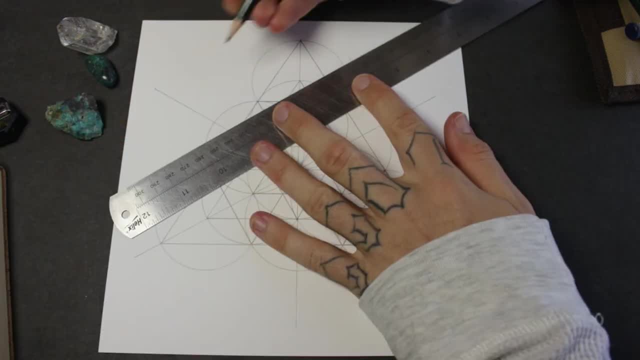 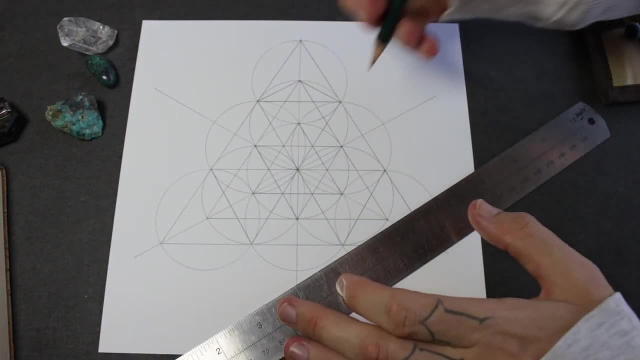 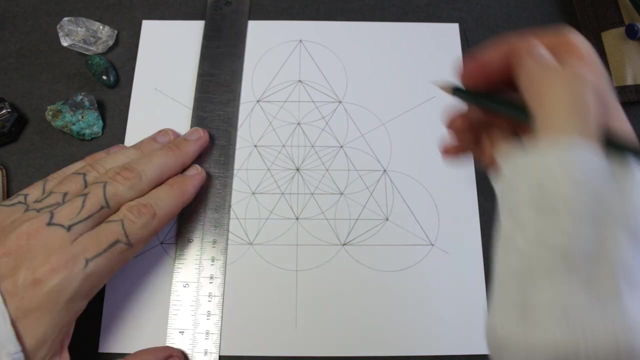 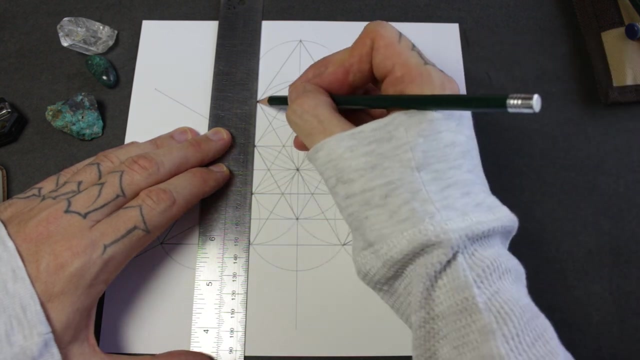 I want to draw a hexagon, So to do that, I'm just going to use all the points of the stars, connect all of them. So I'll start off on the outside And then I'll do one here. This is just going to come down to the bottom of this center triangle. 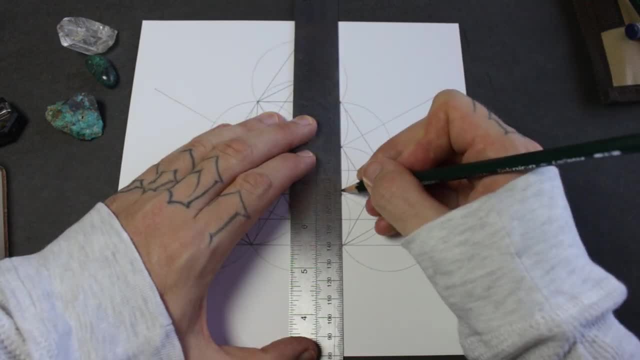 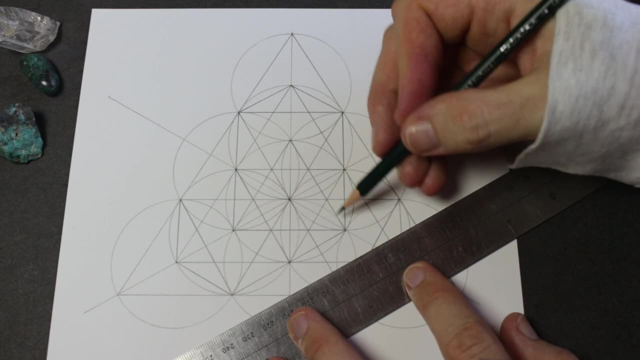 I'll do the same on the opposite side, And then I'm going to do the same, pointing this way: Do that, and then we'll get to the opposite side, Do the same thing there, And then I'll do it here as well. 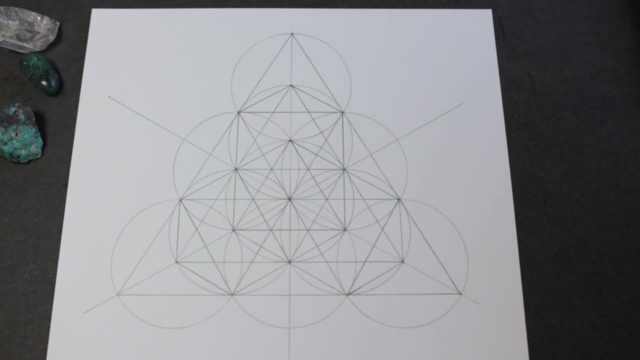 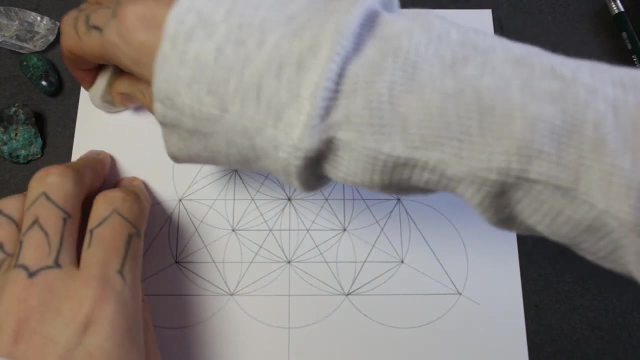 And then that should do it. We've got a hexagon around every hexagram And we've got triangles everywhere, Triangles within triangles. How many triangles, I don't know. Anybody want to count them. Let's rub out these lines that we're not going to need at all. 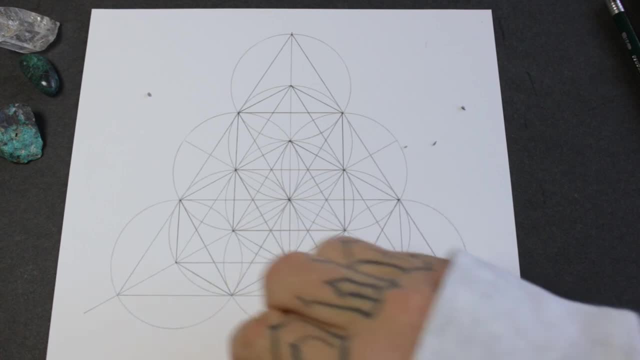 I'm going to keep the circles there, just because I like the way it looks. But these lines they suck, They can get out of you. I'm going to do one and I'm just going to pull off some of that pencil so I can start. 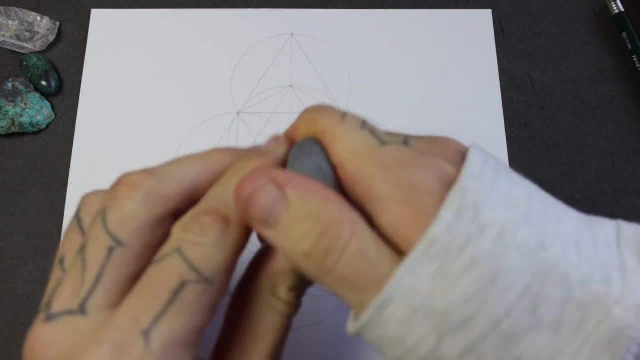 Start going over it with ink. When I'm using the putty rubber, I like to start off with a ball and roll it around, And then eventually it just turns into a sausage, And then I'll just go sausage mode. That's pretty good. 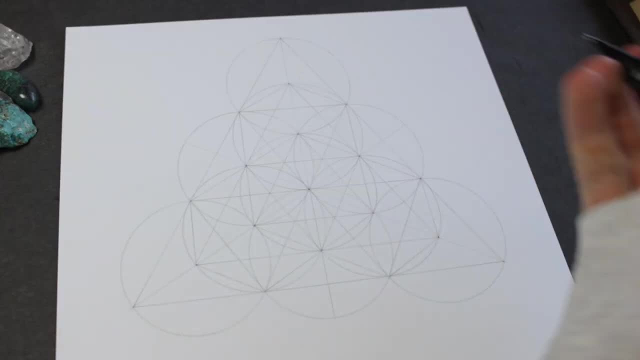 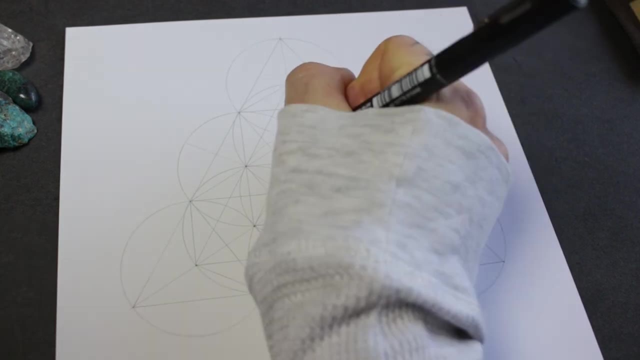 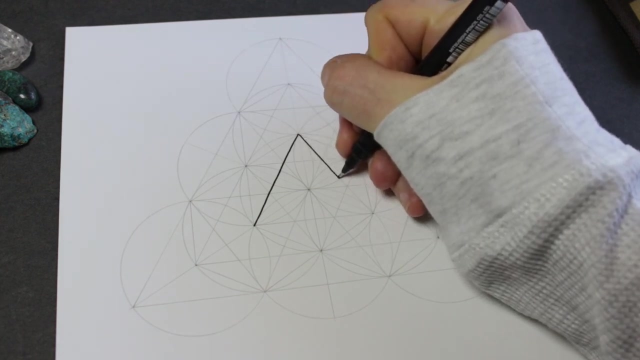 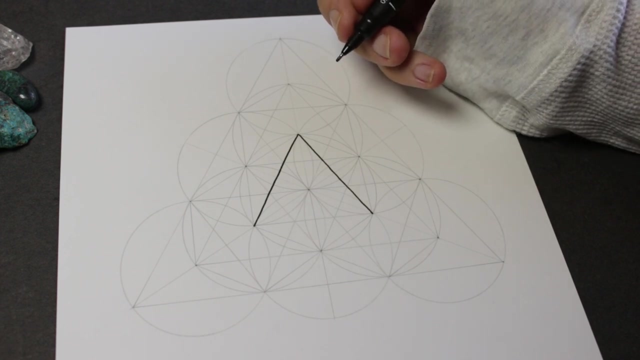 We're ready for ink, So I'm going to start off by drawing in those three main triangles that we did right at the start. I'm going to do it without a ruler. I like drawing straight lines with a well, without a ruler, freehand. 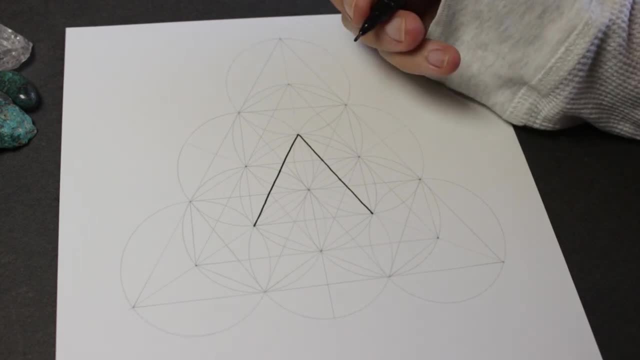 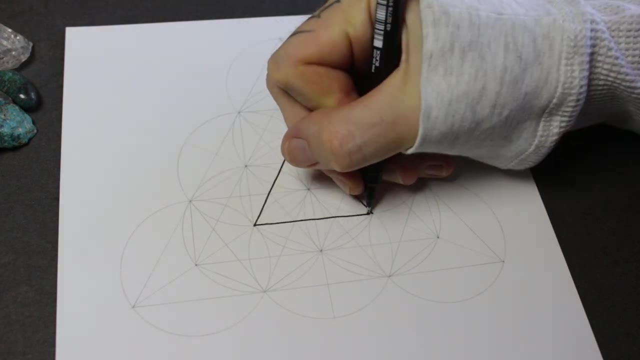 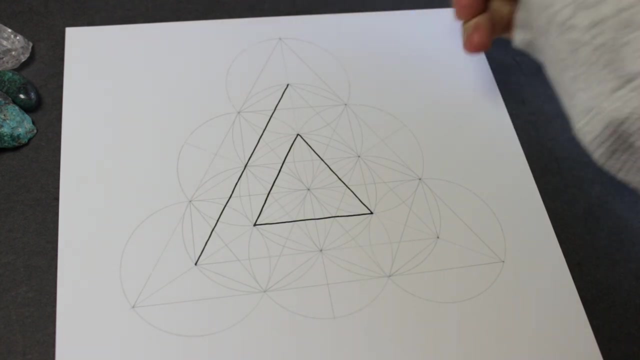 Just because you have to focus on your breath and just really be present, And it's very, very relaxing. Wait for the ink to dry And then I'll draw the next triangle. Focus on the breath And then I'll do the B. 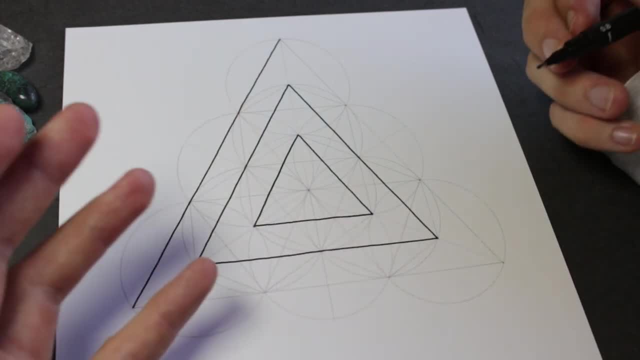 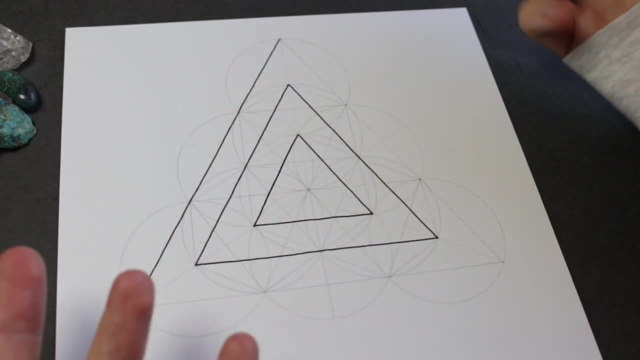 This is the biggest triangle, See. this is the reason why I like drawing geometric patterns. It's not all about how it looks. I mean, it does look cool. You can't deny that it looks cool, And there's something about it that's captivating to us, because it's just everything about nature. 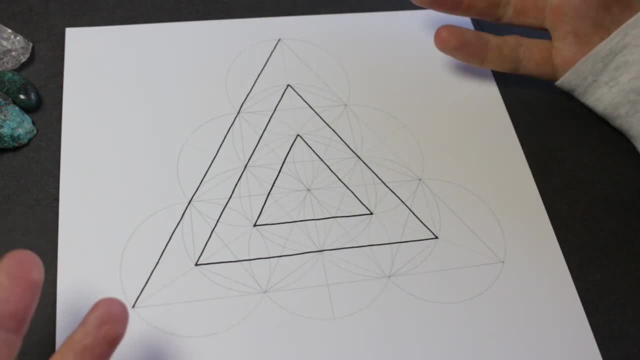 isn't it? But the peace that it gives you. it's like a meditation just in itself, And that's why I like doing it, because it just centers your mind and just calms you. It's just so cool, Peaceful. It's all about the process, isn't it? 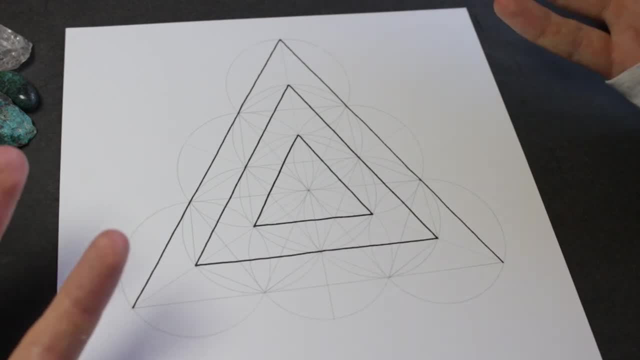 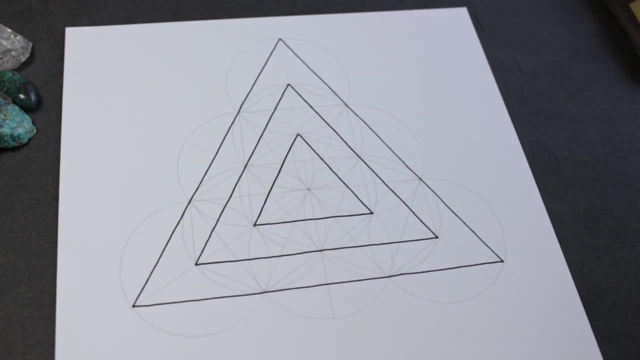 The journey. I guess geometry is like a metaphor for life. It's just enjoy the ride, Don't look for shortcuts. Oh yeah, Looking good. It's good to practice freehand lines as well on paper, because if you ever end up doing, 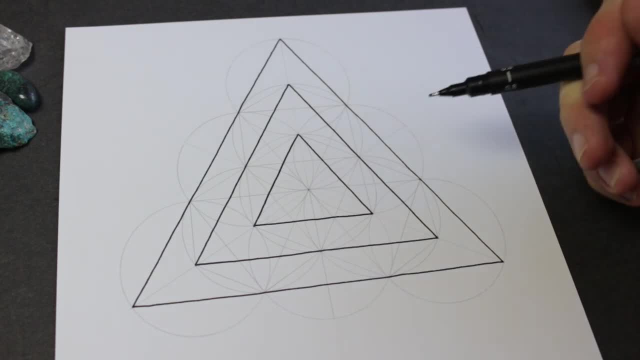 this, doing something on a wall or something, something much bigger. then you've kind of got that muscle memory and the pen control. If you're doing it with a camera, you're doing it with a pen. If you're doing it with a can, it's the same. 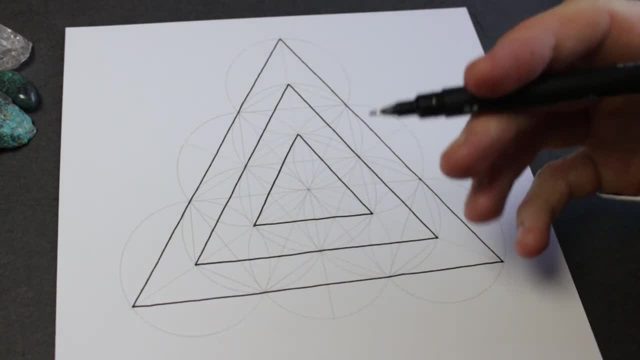 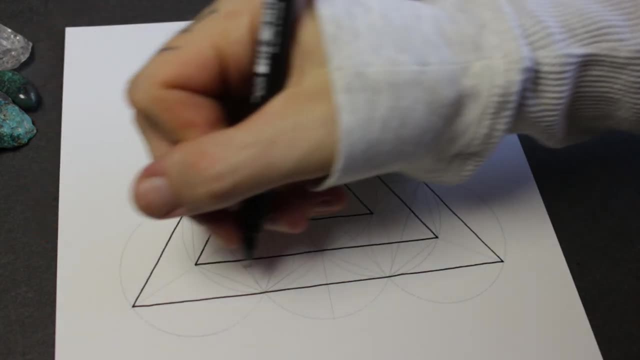 You know you've just got that control because it all comes from your shoulder instead of the wrist. When you're using a ruler, you're just doing it all with your wrist, But when you're drawing a straight line, it's your shoulder that's moving. 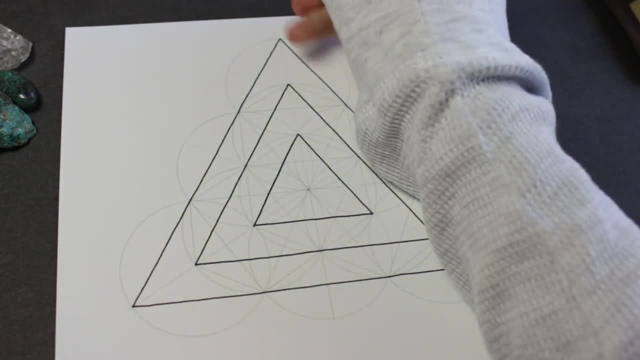 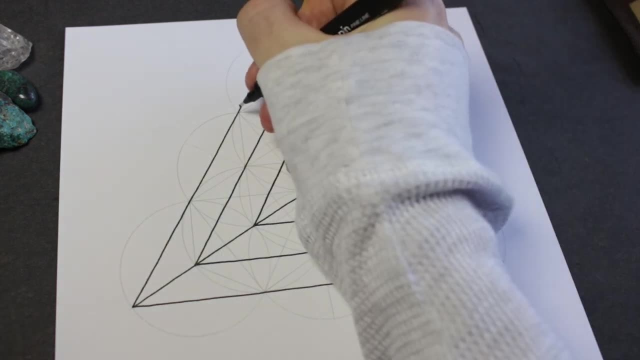 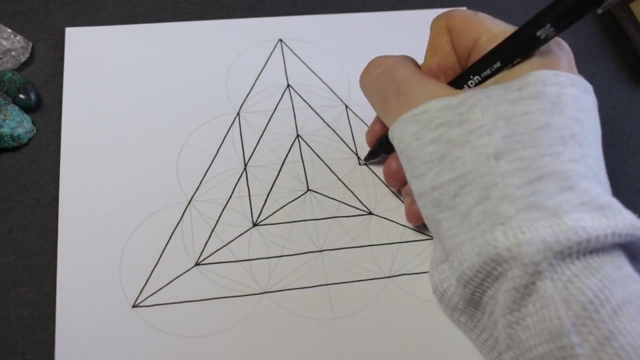 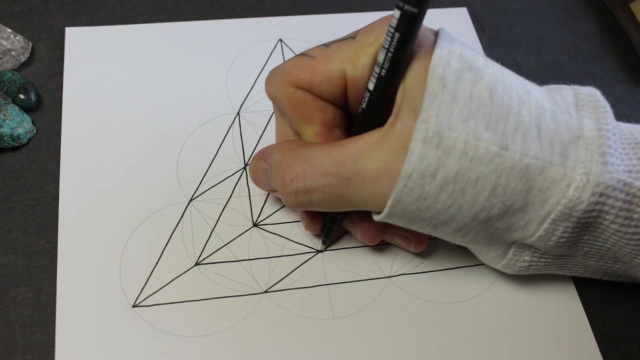 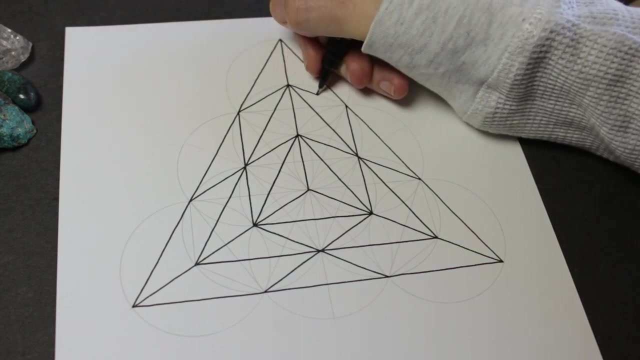 Now I'm going to draw. I'm going to connect the tips of the triangle to the center. Next up is those lines that we drew for the hexagons. I'm going to add those lines to each side of the triangle. I'm going to draw an arc in the middle of the triangle. that. 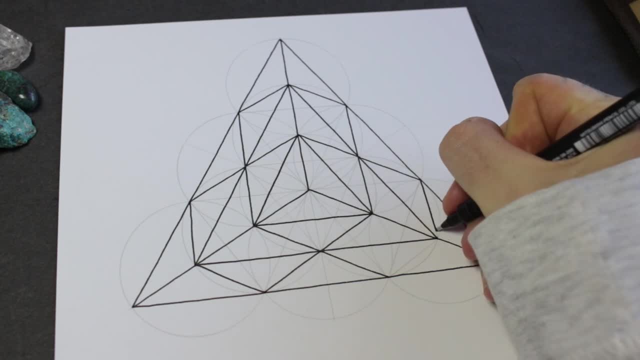 I want to make a circle, Then we're just going to connect that to the hexagon And then I think this is close to the end now. I got to draw the triangle on the top, The first thing I'm going to do. 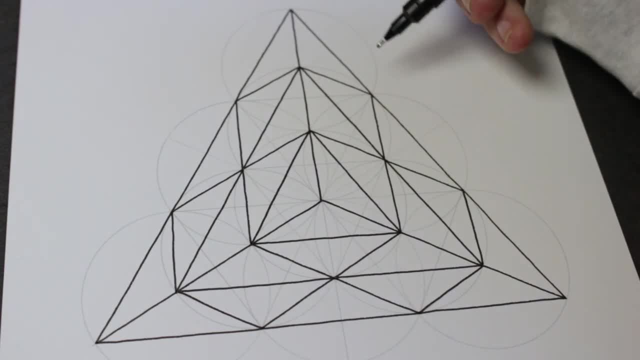 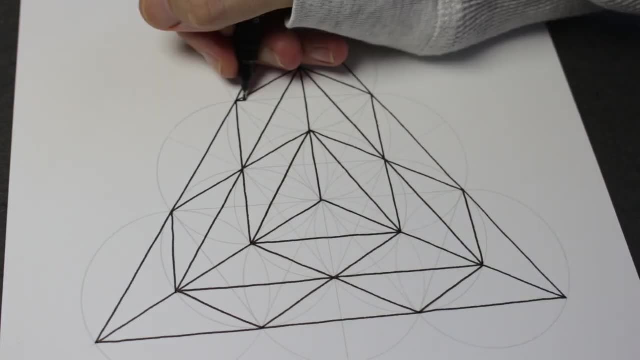 I'm going to do a very small line The size of the triangle. Then I'm just going to connect the dots points of the hexagrams, but they've got to be sitting behind the triangles that are pointing up. so hopefully I get this right. 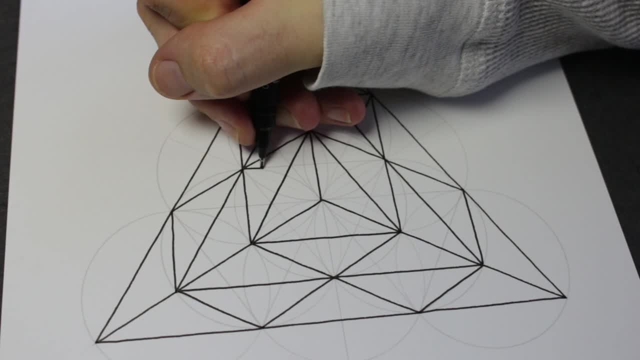 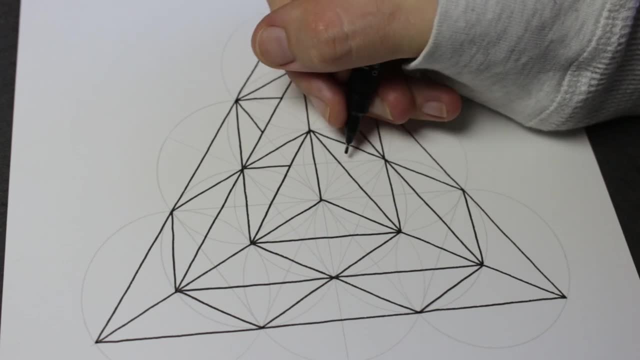 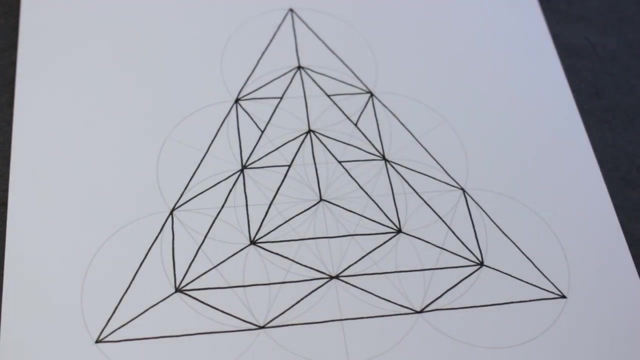 and then this is the triangle that points down in the center and it makes kind of almost like a star tetrahedron. I mean, this whole pattern is very similar to the 64 star tetrahedron. I'd like to see what this look like in 3d, to be fair, because it's- I don't know it's.